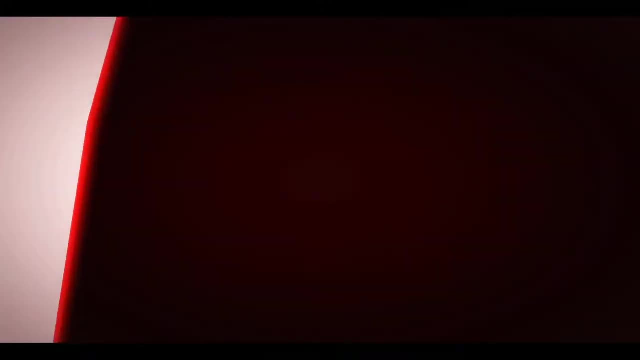 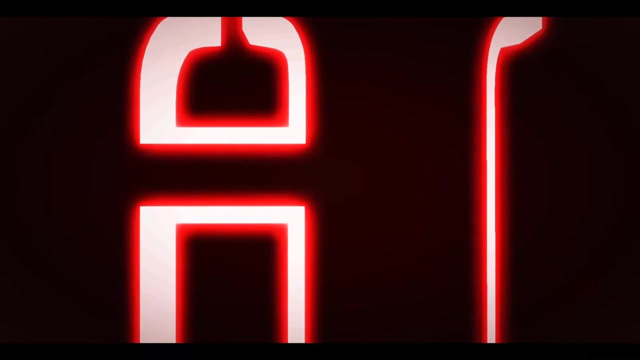 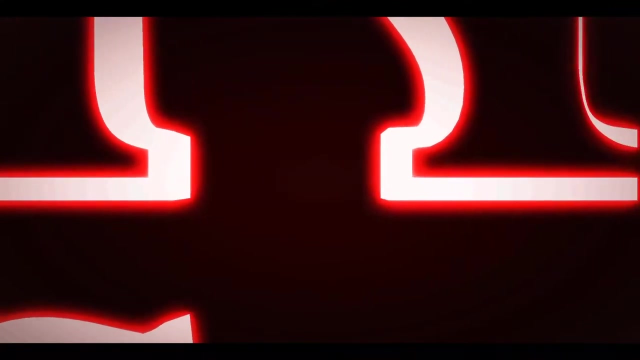 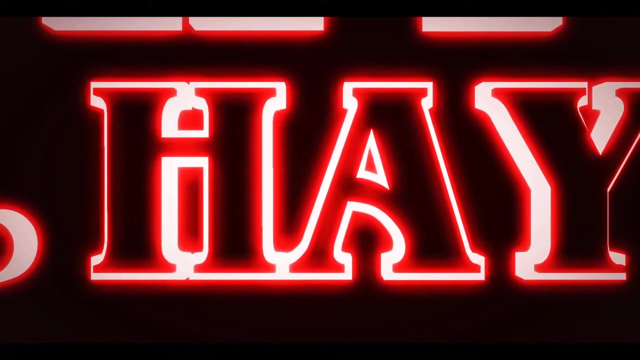 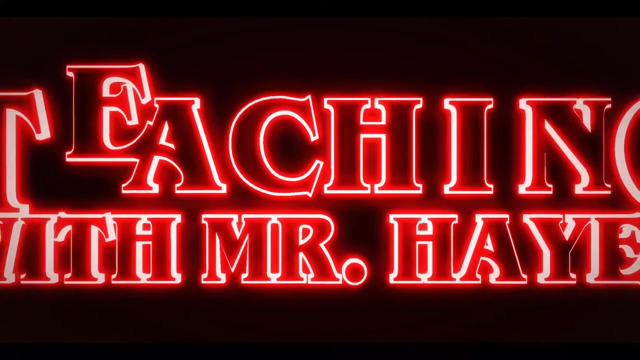 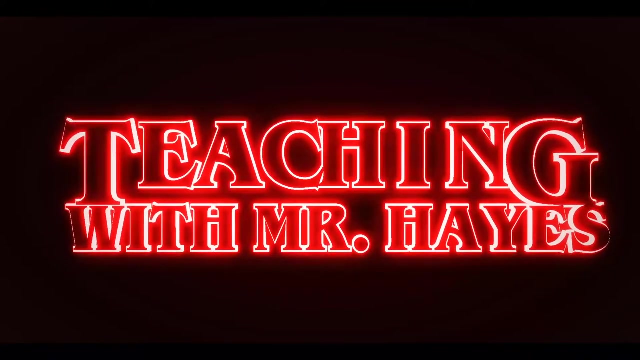 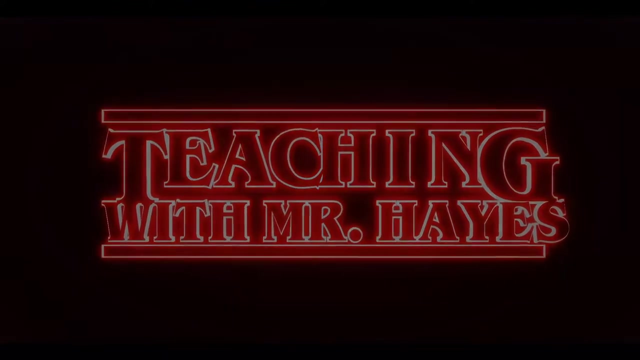 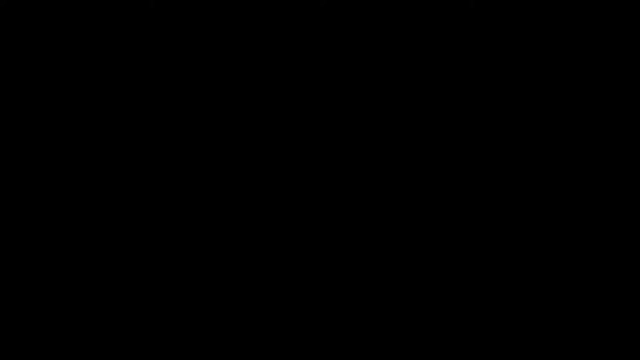 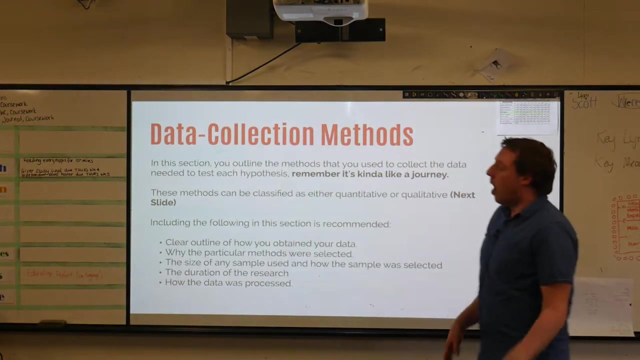 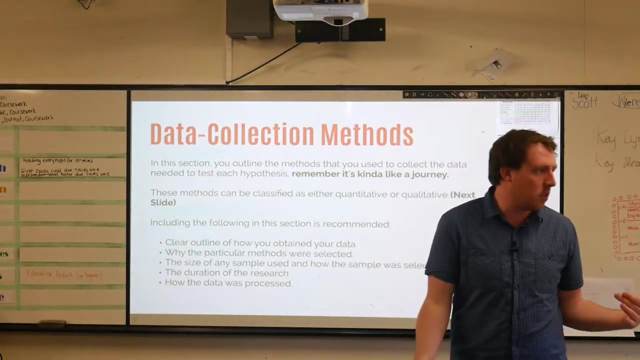 Thank you for watching. Thank you for watching. I'm also going to put this information into that Word doc that I had shown you yesterday so you can use that as a point of reference if you're working on it next week. But Friday, fingers crossed, don't give me a relief. 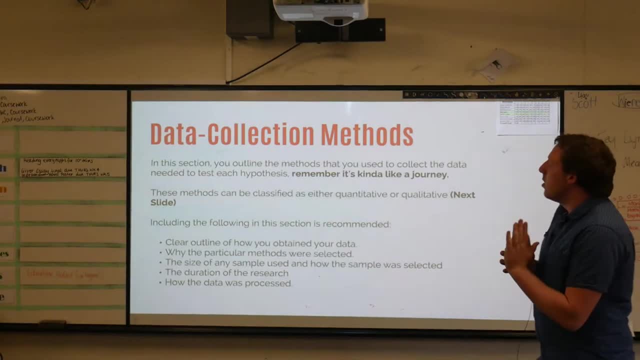 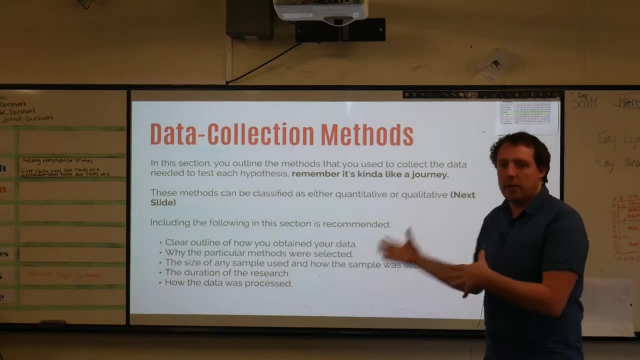 I'll pull you back out and we'll have our classes as per normal. So in this section, basically, you're outlining the methods that you use to collect the data. You've got to treat this as a bit of a journey. So many of you- we all- went on a journey to collect our data. 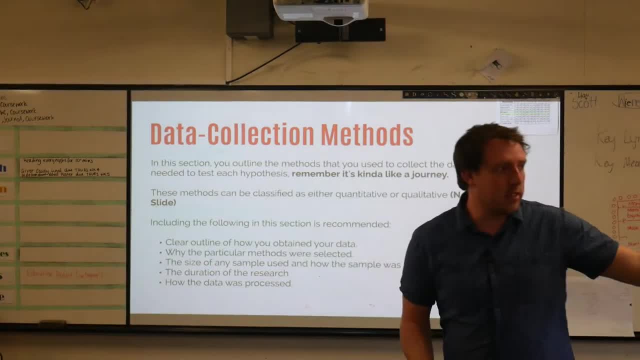 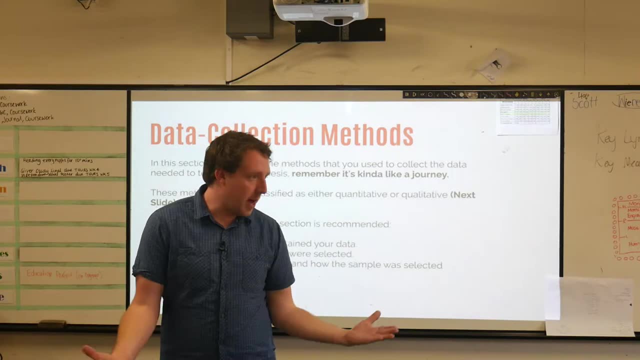 We started on a very hot Wednesday going around the school picking up the rubbish. We used that as a foundation for data. Then, the next lesson, I got you to grab maps And you mapped out where you thought the hot spots were for that rubbish. 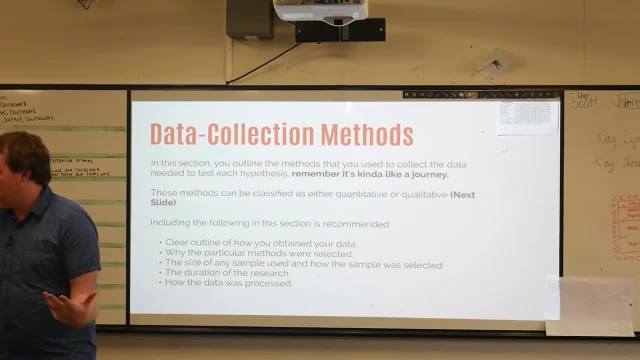 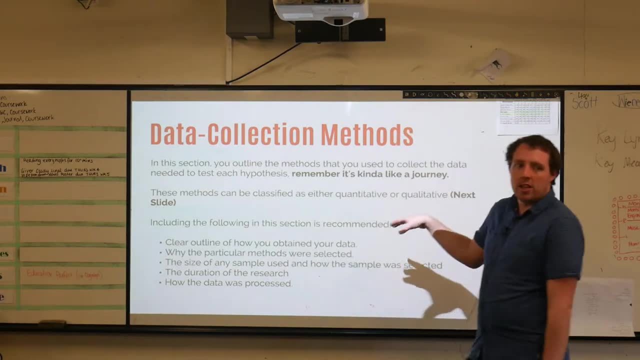 And then the other day, you then decided your third set of data, your own data. So some of you did surveys, some of you have done an interview, some of you went out and collected rubbish. I want to see that journey in depth, in detail outlined. 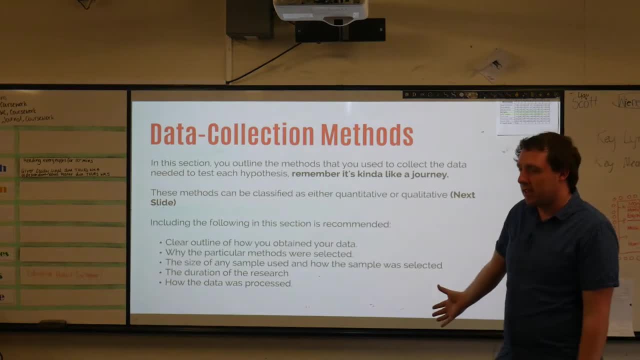 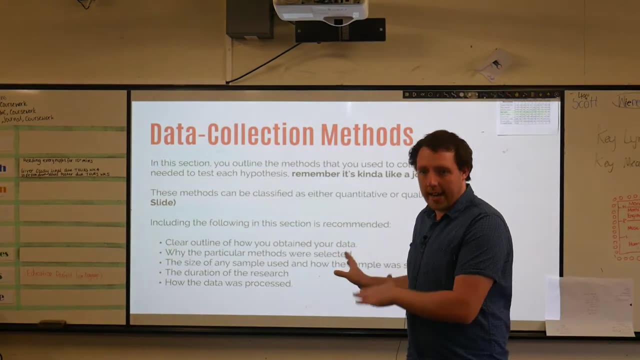 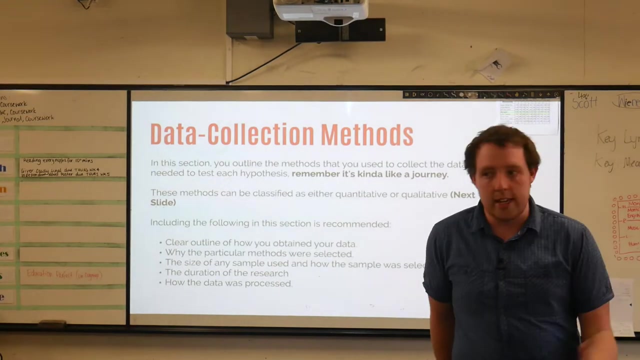 Think of it When someone's reading this. it's important in a field report that what you are presenting is true and accurate And you have actually properly found that data and you're just not talking about random stuff. So it's really really, really, really important to really go into depth and explain that journey to me. 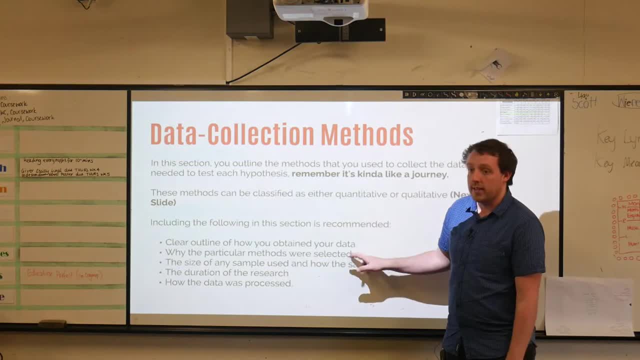 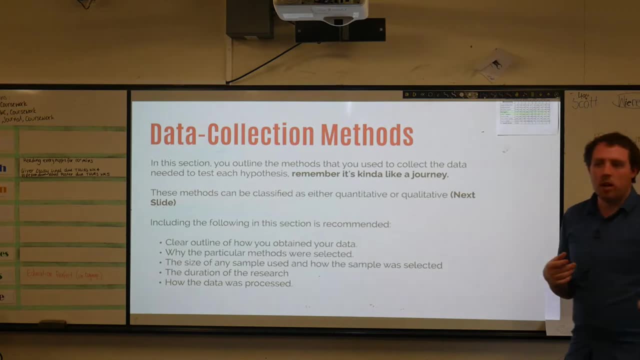 Well, you can just write down this kind of stuff here. So include the following in this section. Make sense, So also you also need to. I'm going to use some geography terminology. Hopefully. have you guys heard of the word quantitative and qualitative before? 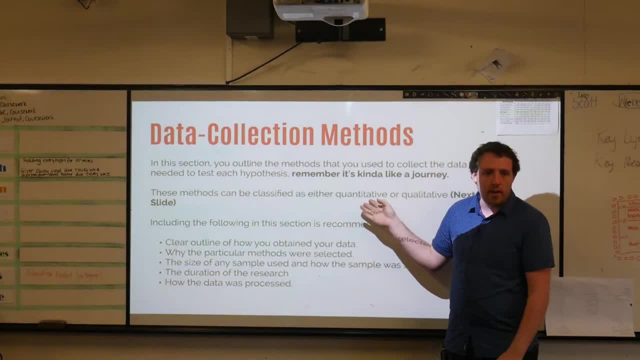 Surely Yeah. so quantitative- What's quantitative? Annalise Can't remember. Jesse, Do you remember what quantitative is? No, anyone remember what quantitative is? Will? Yeah? so guys remember when we went out the front and we watched cars go past with Ms Cote? 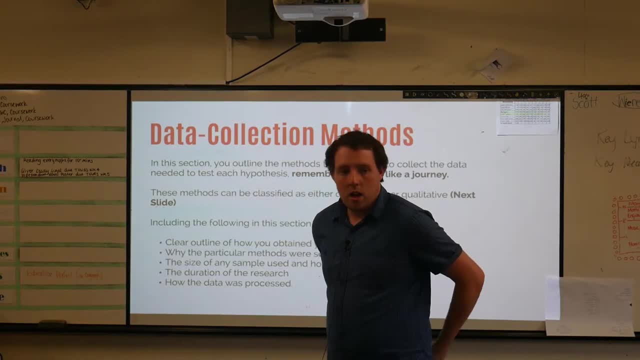 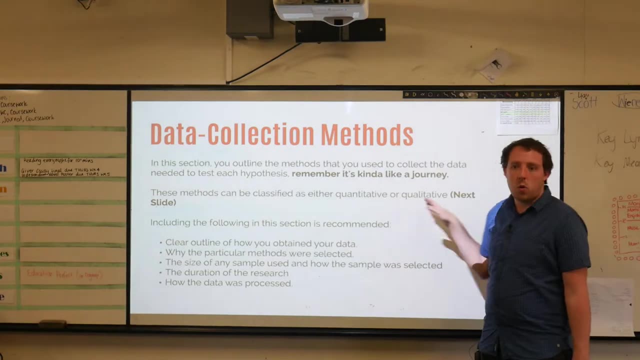 It was about what kind of data? Yeah, One's categorical and one's numerical. Yeah, so quantitative is very numerical, It's based purely like numeracy, okay, Whereas qualitative- So quantitative- is your surveys, okay, Where you go out and you say yes or no. 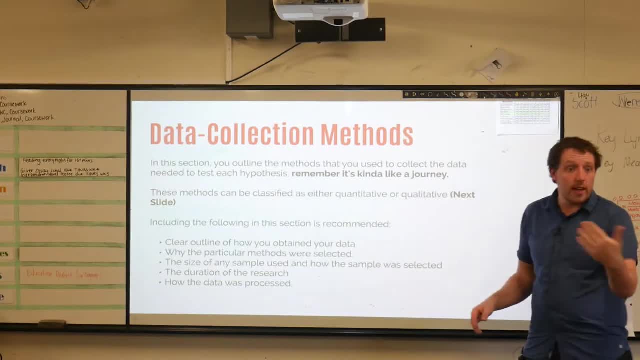 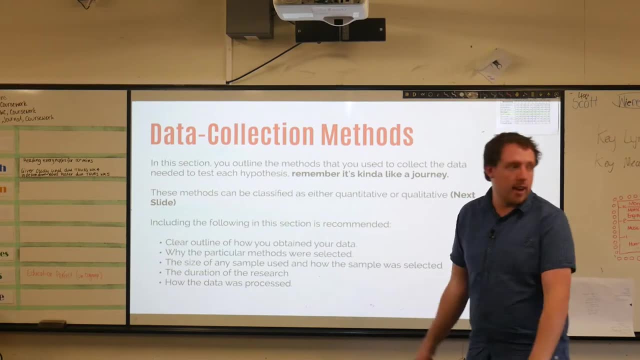 They're a form of that, Whereas qualitative is your interview. You interview me and Will. that's qualitative, All right, Does that make sense? So there are two very different set of data. There is a slide that explains it after this. 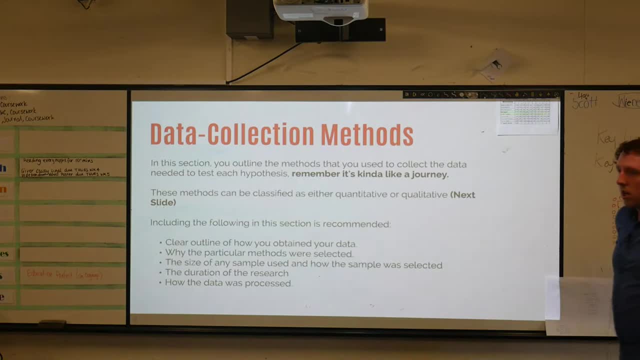 But Qualitative is like quality, which is why Mr Hayes and I were giving interviews. Yeah, Because you want quality interviews. Well, I got interviews, So did I? Yeah, so we're Even before you. Well, do you know what? 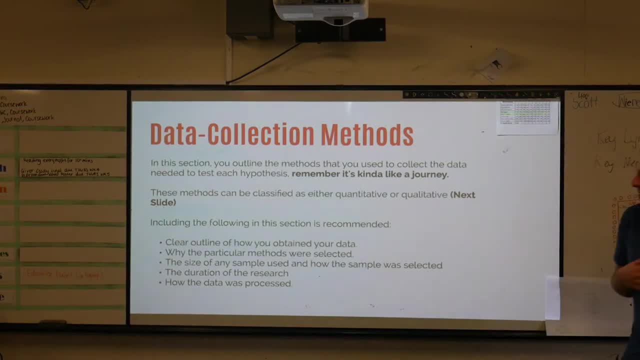 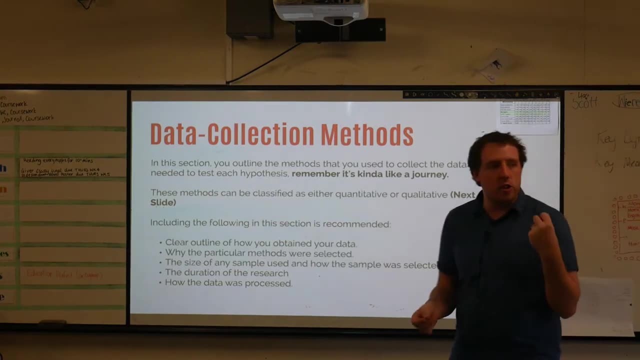 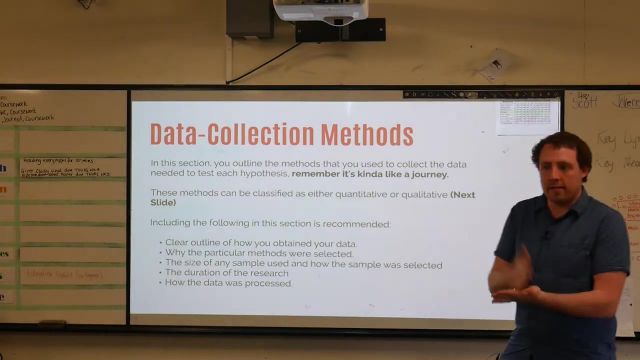 You suck. Give me the background. So you want to include the following in this section? So clear outline of how you obtained that data. It is a journey that we- I would love to join with you. You need to be able to explain to me. this is how I got my data. 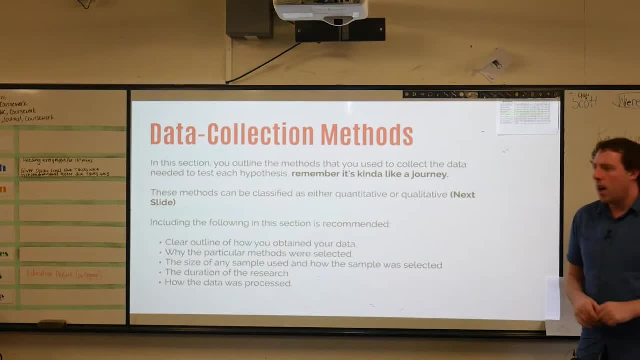 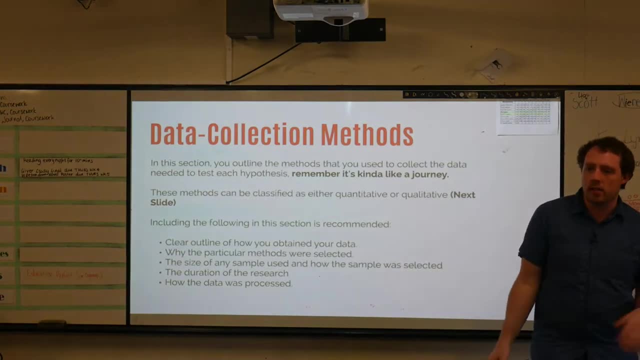 Break it down step by step. Right, I did this, I did that, All right. Also, it's really important to explain why the particular methods Were selected. So, for example, Liam, you decided yesterday to go around and take photos of the rubbish. 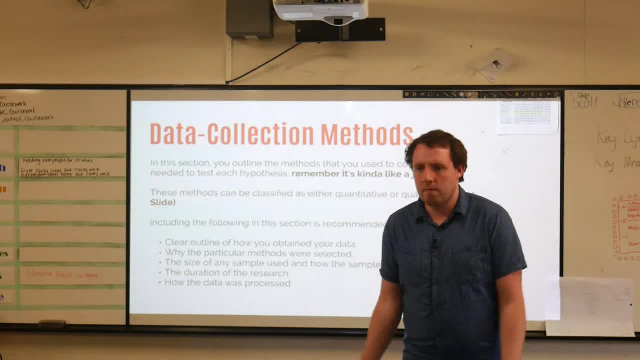 didn't you? Why did you choose to do that? What's the reasoning for that? So you can see, like, how much rubbish is in the survey area. Yeah, excellent, So that's what you include. Liam's, then provide. 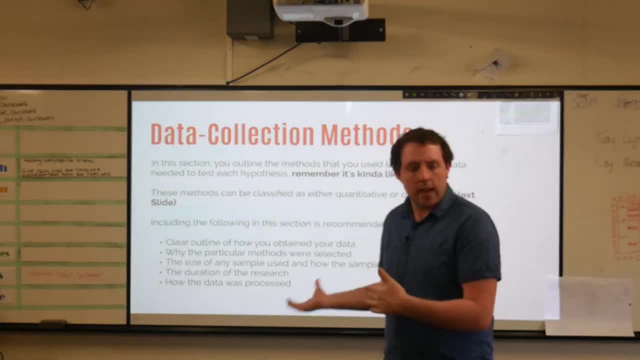 Obviously, you probably want to go in a little bit more depth, But Liam has just said to me: well, that's why I did it. Okay, So that's why you include. Why did you interview Will and I? So I can clarify things. 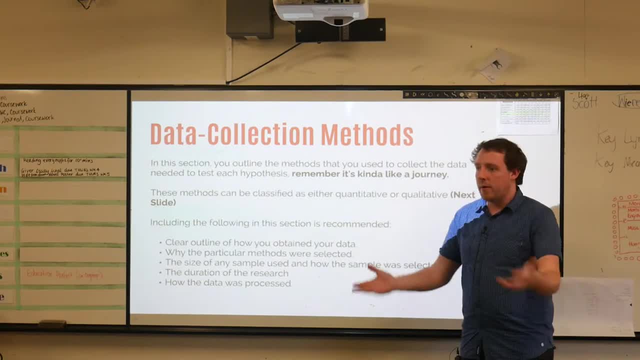 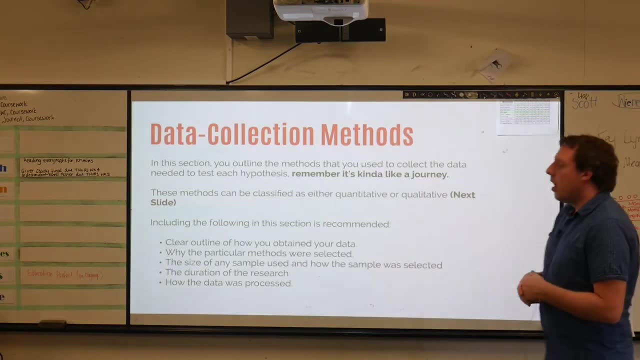 Yeah, Cool, You write that down, Same with Yaron and Sophie. You guys did your survey, So why did you? That's what I want you to tell us. Okay, In your report, All right, You also need to note that. you know, for example, you also might want to say like: 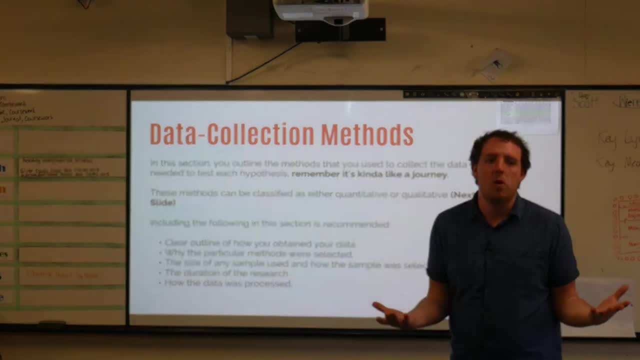 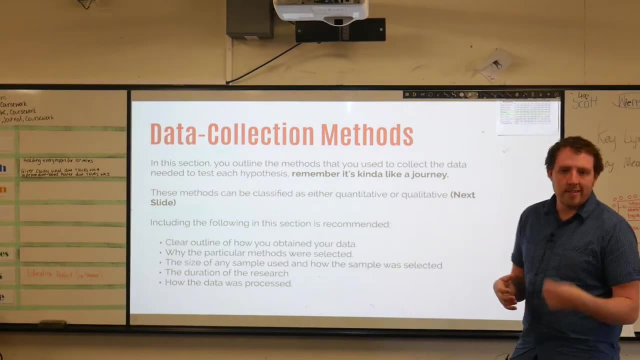 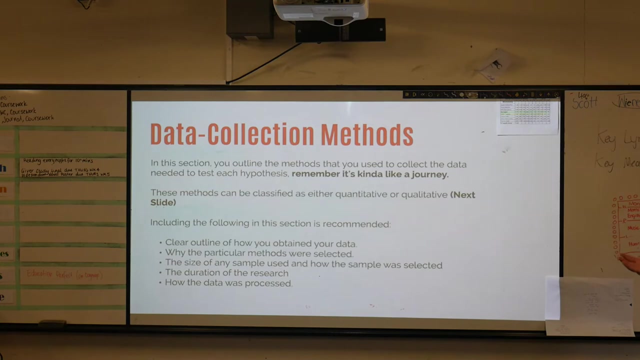 I did a survey because I was able to survey 25 people who gave me a wide range of points, perspectives, viewpoints, etc. Those are the kind of reasonings and explanations that I want you to include. You also really want to talk about the size of any sample used and how the sample was. 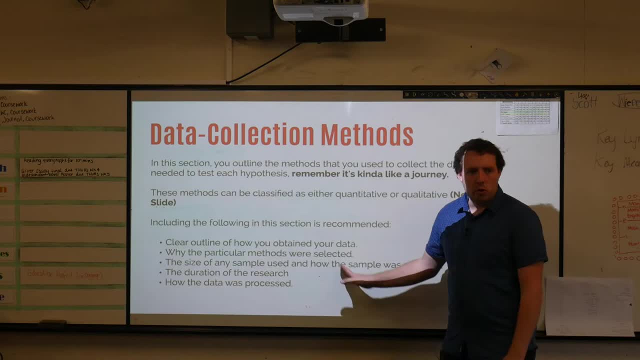 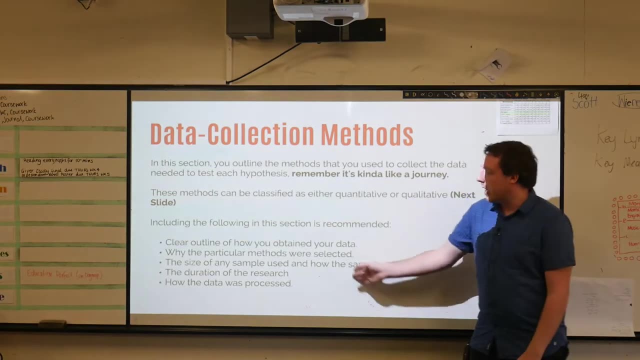 selected. This more so applies to people that took your surveys. All right, And really you and Hayley did, didn't you? And so far, Sophie and Yaron. So really, here this is more going well. how did you select your sample size? 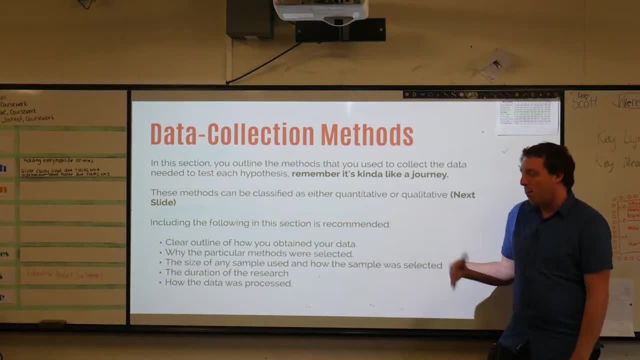 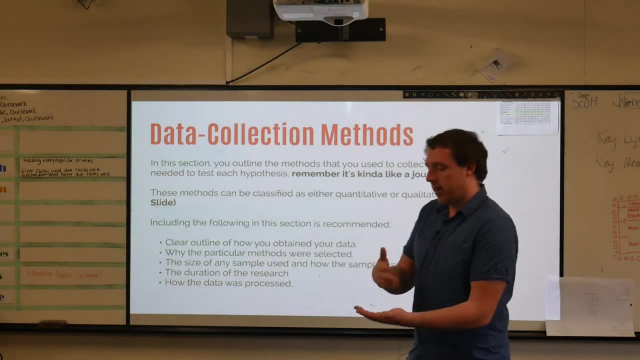 So how big was your sample size? So that's how many surveys you handed out. Why did you choose that sample size? And also how the sample was selected. So you might have gone. you might say: well, we targeted year 10s, year 11s and 12 students. 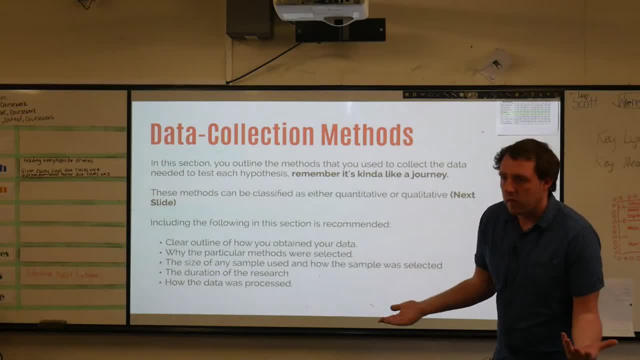 because we wanted more appropriate, mature responses. Okay, So that's why your sample size was selected like that: The duration of the research, So outlining how long this research has gone for, And it's probably gone for two weeks, All right. 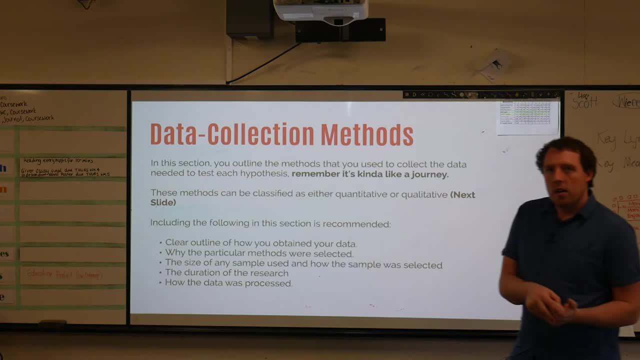 We spent maybe four-ish lessons- I would say Not even that- Collecting all your data, all your research. So you talk about that, Okay, And then how the data was processed. So if you've taken photos, you would say, well, we've analyzed the photos. 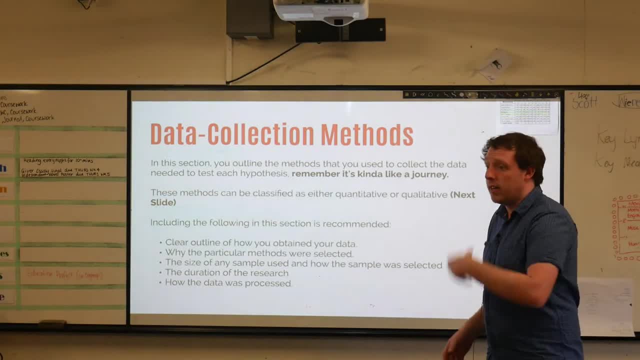 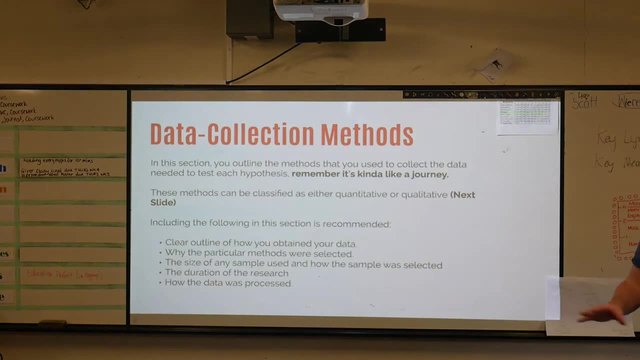 We've talked about them. If you've done surveys, you might say, well, we've actually graphed them. You might say, well, we've actually graphed the surveys. All right, You also with the initial going around the school, you can talk about how we mapped out. 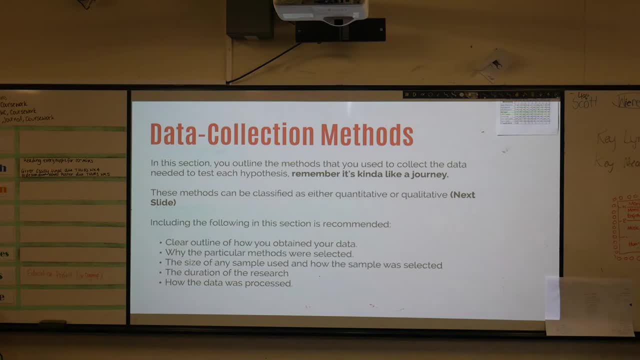 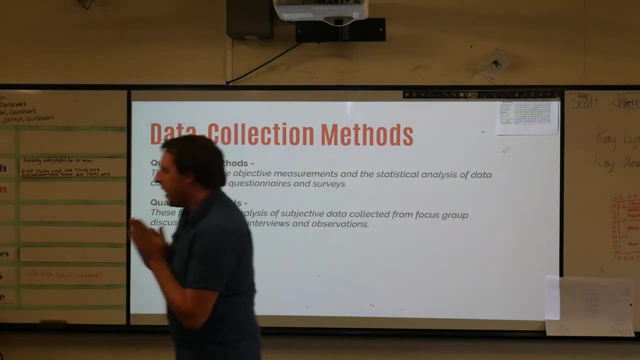 the different hotspots in the school as well. All right, Does that make sense? I will put these all in a Word doc and I'll explain them as well, So you can use them as guiding sentences. So data collection method is, we have quantitative methods. 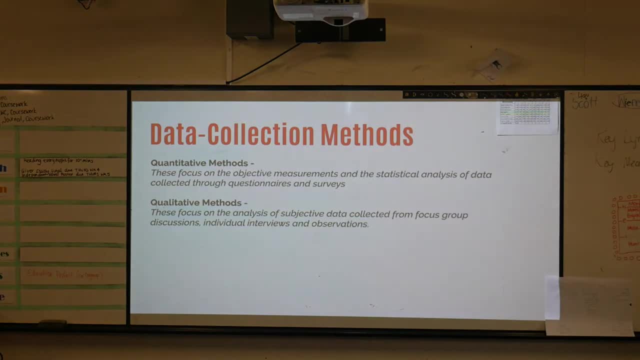 These focus on objective measurements and the statistical analysts of data collected through questionnaires and surveys. All right, That's focusing a lot more on the numerical side of things. Qualitative methods: These focus on the analysis of subjective data collected from focus groups discussions. 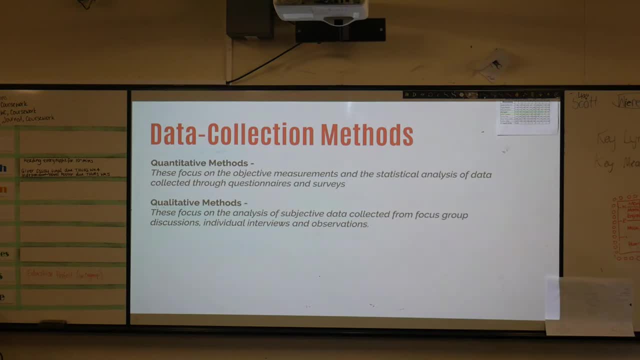 individual interviews, observations. So, for example, you've got Brianna to go around Qualitative Okay, Because she's observing people. She's not necessarily getting stats, She's just observing people, taking notes and going okay, cool, cool.